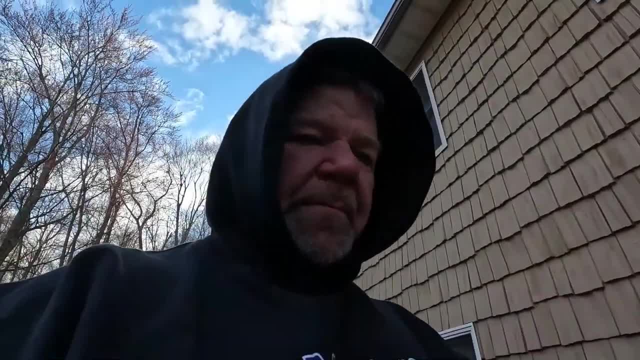 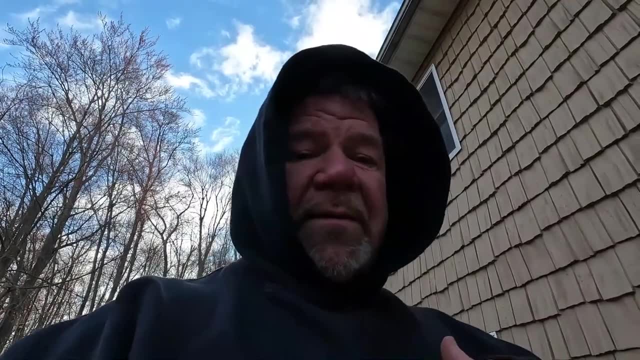 put it in a bag and we sample it on our PID meter That detects the hydrocarbons, or in other words the extent of the contamination. We use that as a start point. So we sampled this and it was 685 tons of soil. That's where the contamination begins. So we dig down to where the 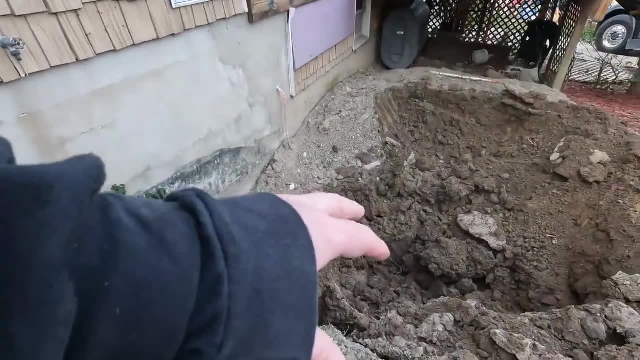 contamination begins. So we sampled this and it was 685 tons of soil That detects the hydrocarbons, or in other words, the contamination begins. So we sampled this and it was 685 tons of soil. So we'll continue to remove the gray soil until it gets down to about 30.. When it gets. 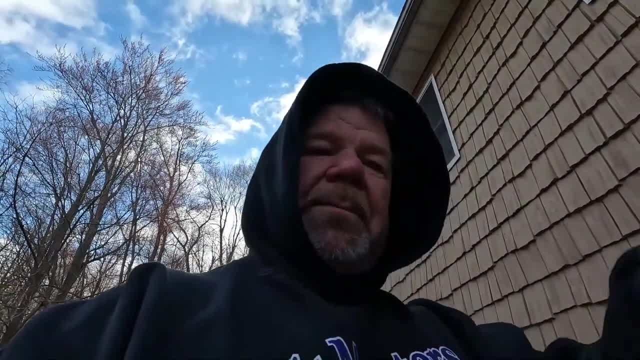 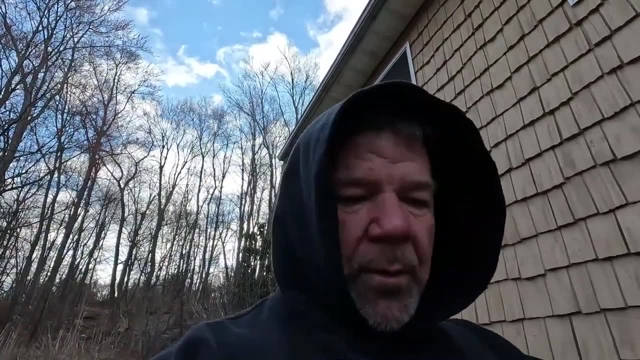 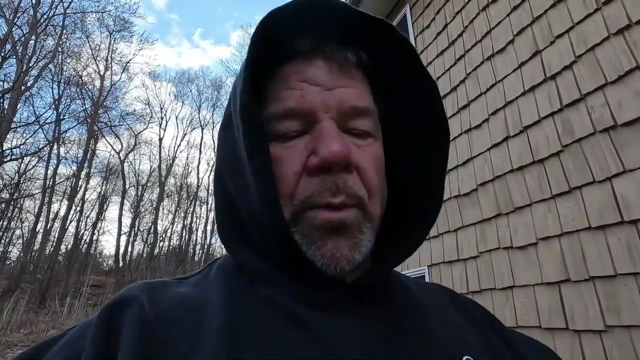 30 on the PID meter. I know I can then take my post-excavation soil analysis. That's what the state requires in order to remove the case or the spill number, And we just go based on that. That's what determines when we stop digging. 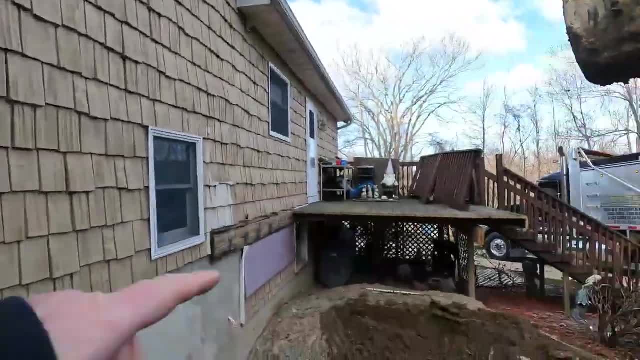 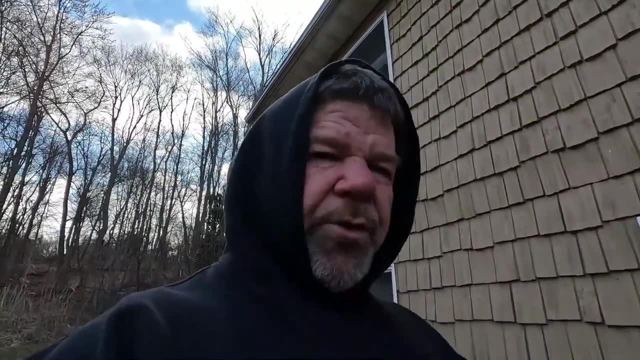 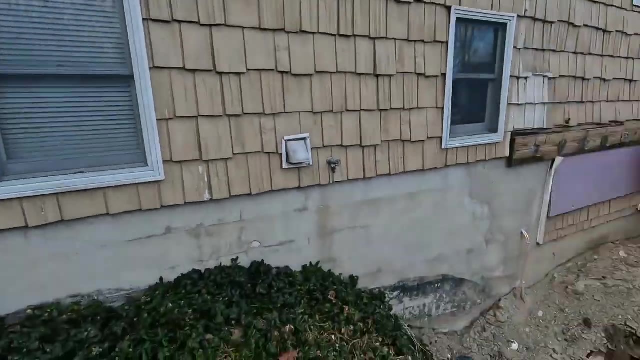 Once we get that schedule date, the day we come out, we set out all these ground protecting mats, we go over the scope of work with the homeowner on where we're going to sit, where the trucks are going to sit, what we can and what we can't do, based on the permission of the homeowner. so then, when we come out, 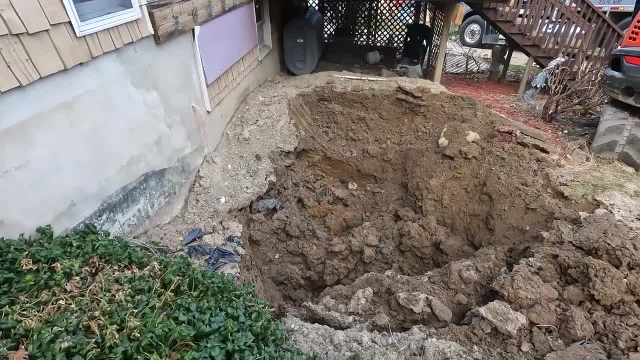 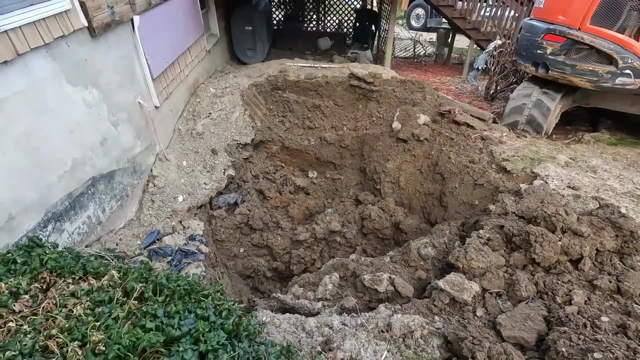 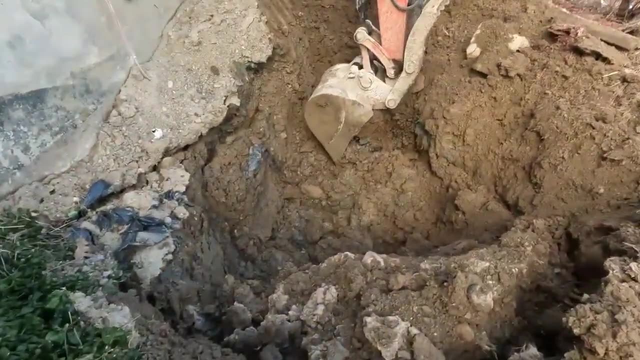 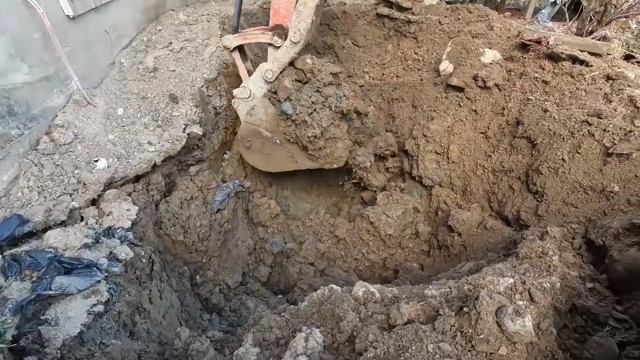 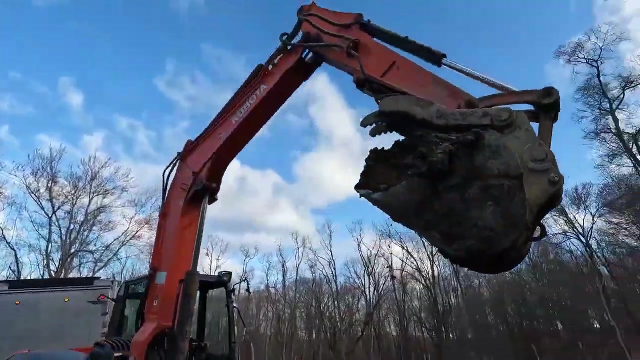 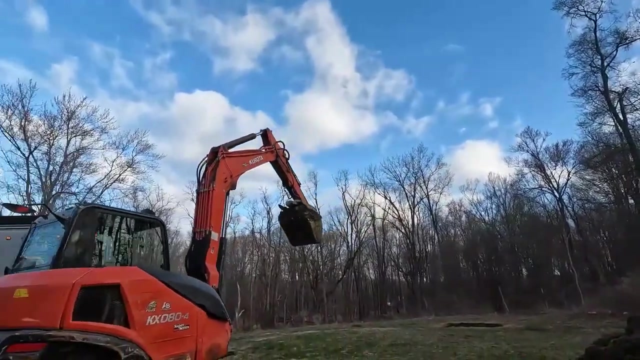 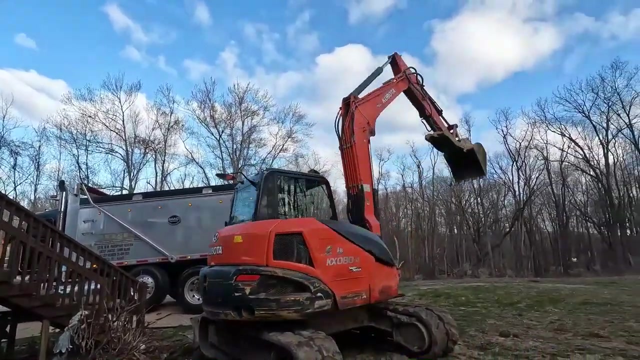 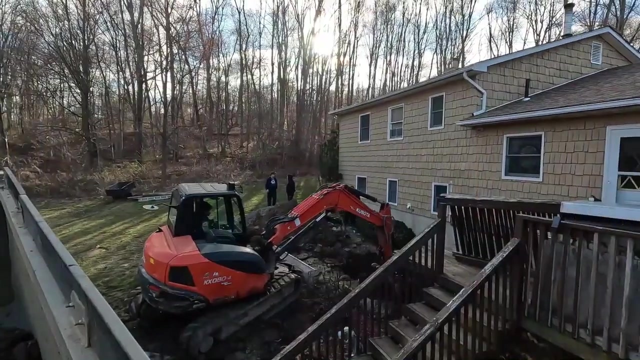 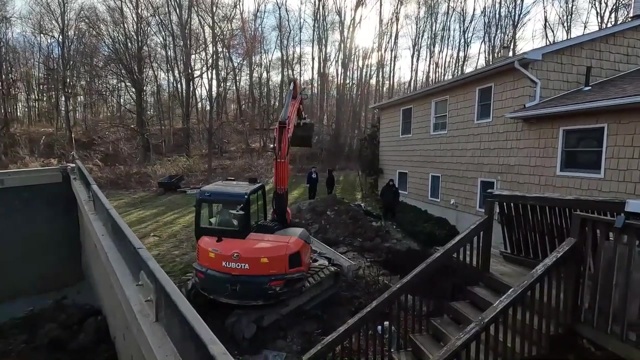 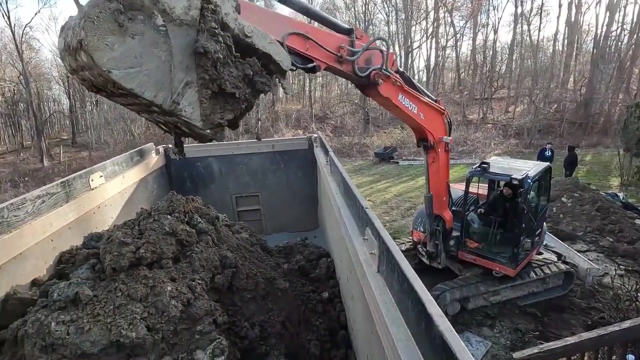 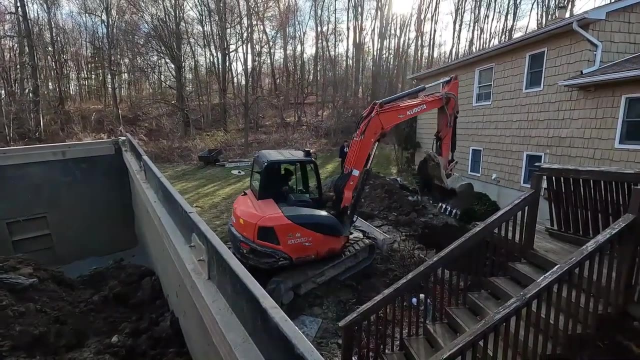 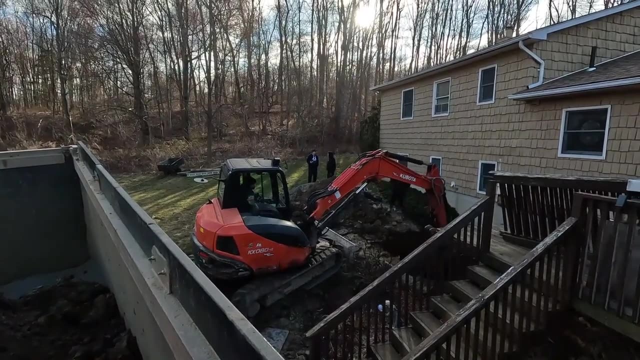 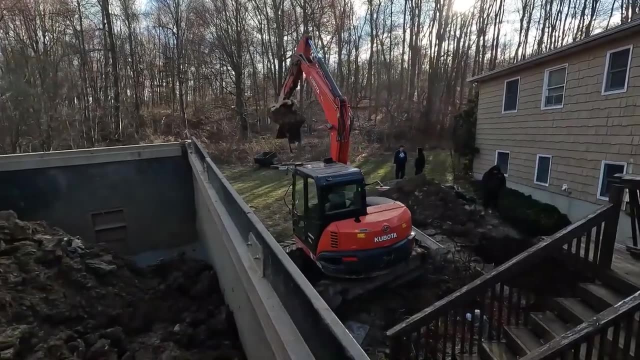 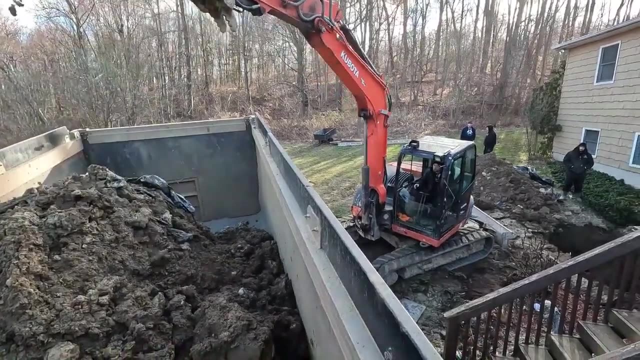 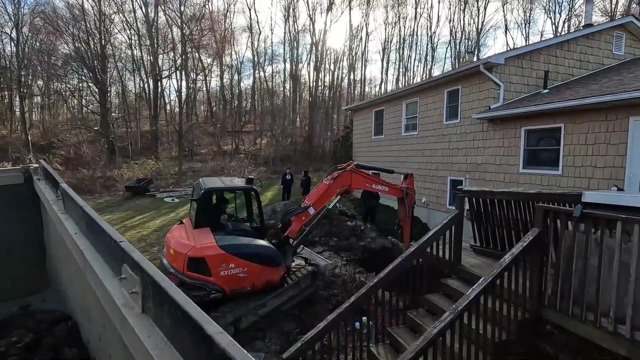 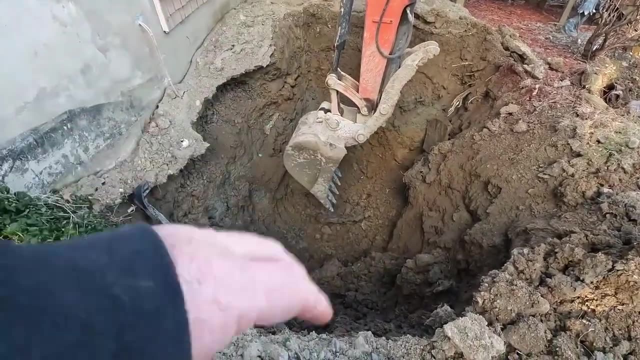 we take that start point reading with our pig meter and we just begin to excavate. we'll dig down about six or seven feet, and then we'll take another pid reading, and then we'll take another pid reading, and then we'll take another pid reading. throughout this process we're constantly screening as we go. 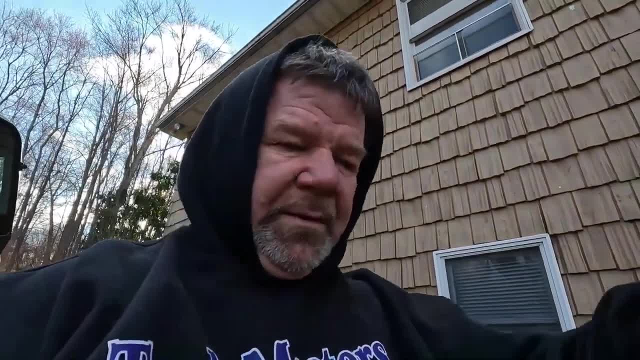 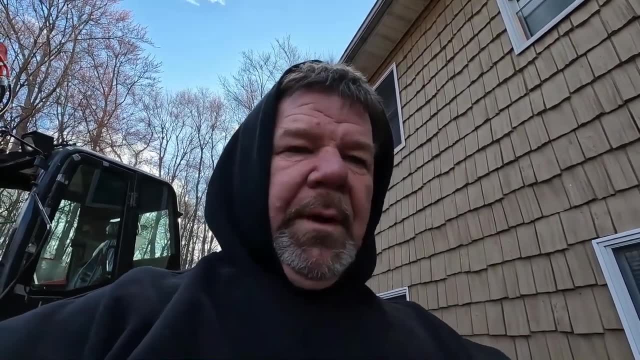 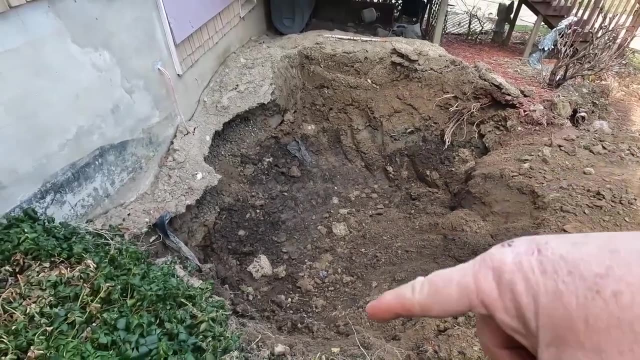 so once we remediate all the contaminated soil, the DEC knows that we've cleaned up this site when we give them a clean bottom sample right here and then four clean side walls. now there's the two sides of the site that we've cleaned up. two ways we take these samples is called a grab and a composite. 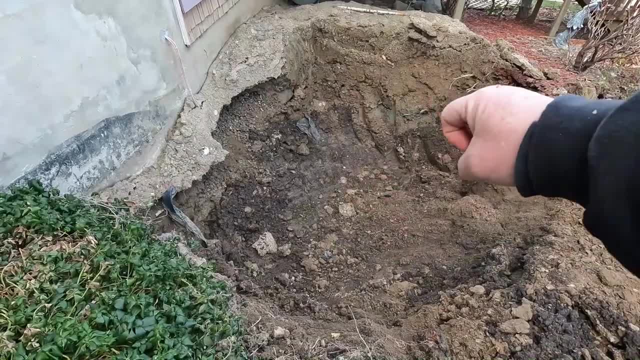 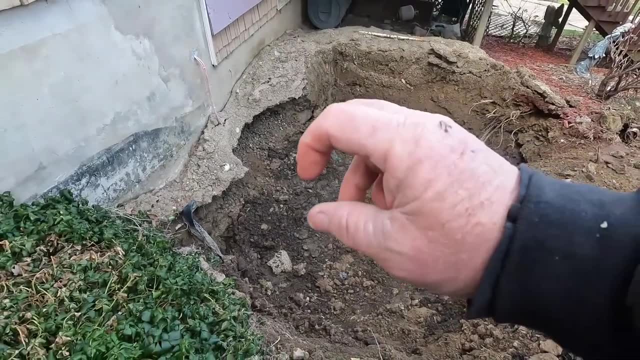 that center bottom is a grab sample. we just grab it, we put it in a jar and we send it to the lab. it gets sampled. the four side walls are a composite, so we grab a little from that side wall, grab a little there, grab a little there, grab a little there. 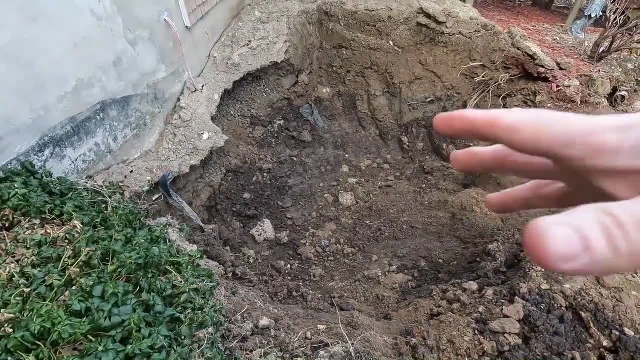 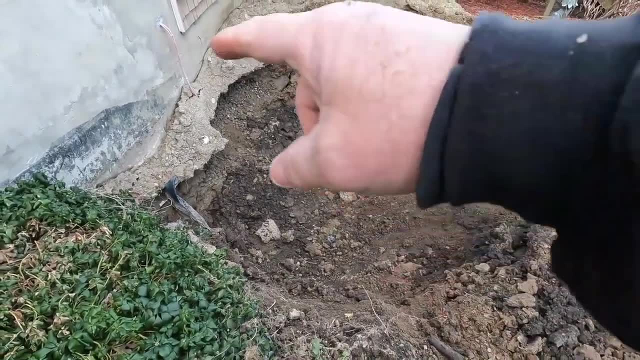 we put it in one jar and that's a composite. so in order to once this area is cleaned up, those are our post excavation samples. we take one bottom grab sample that we put in a gal and a four side wall composite, and we've done that already and took the readings. they're all. 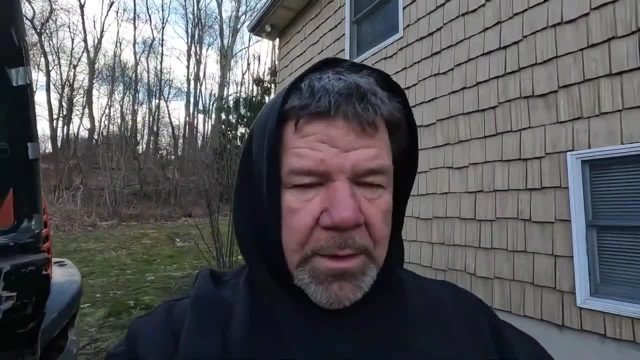 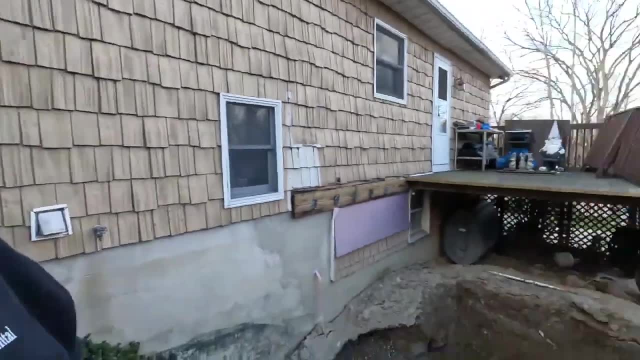 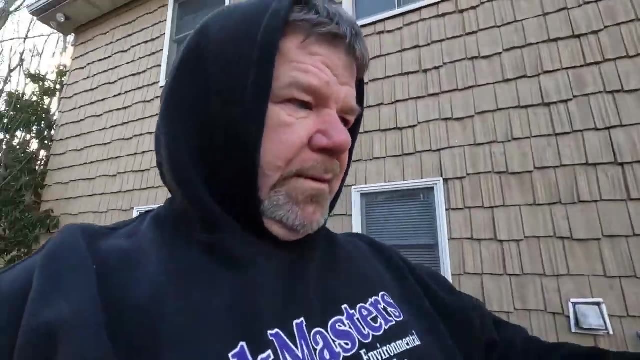 acceptable. so once we've taken our clean samples, we then put back the overburden- it was about seven tons there- and then we backfill it with a item crushed that minimizes any of the sinking. they're going to put a patio back here, so anytime i go beyond. 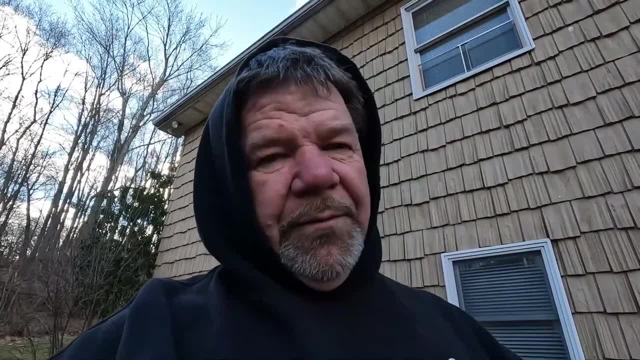 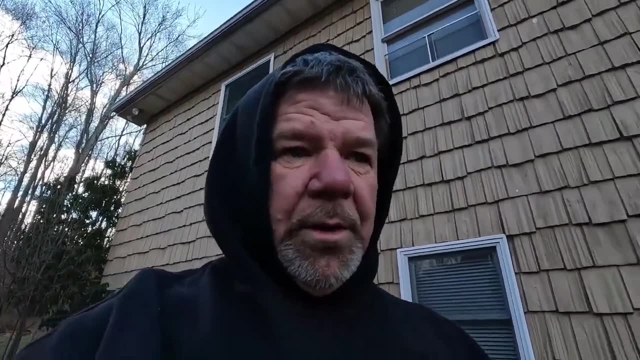 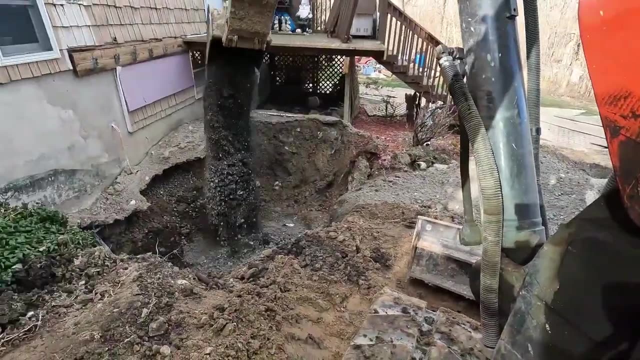 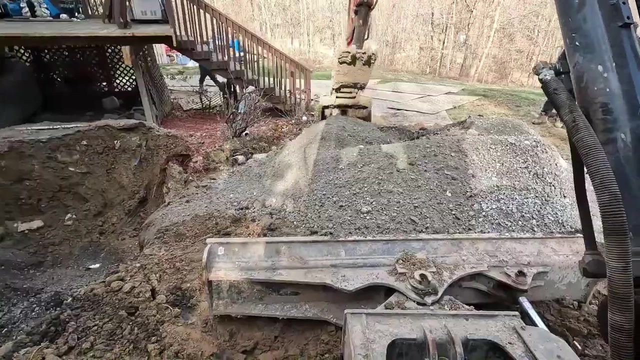 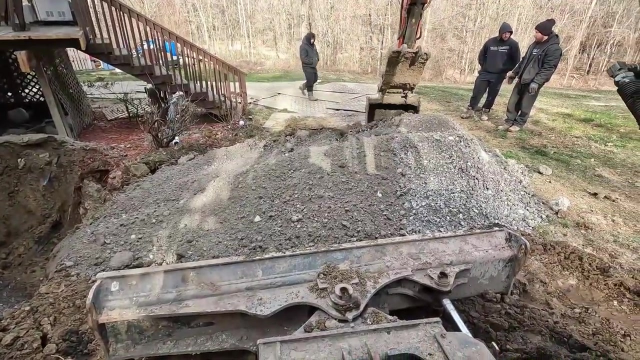 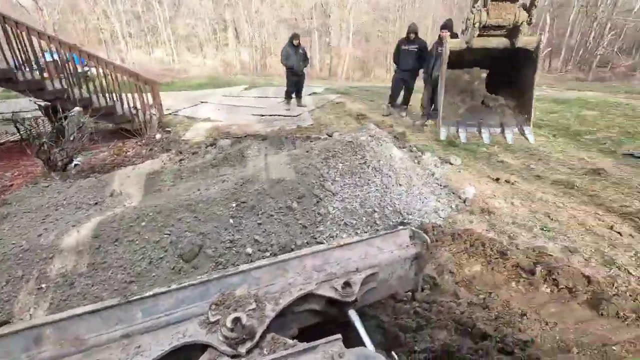 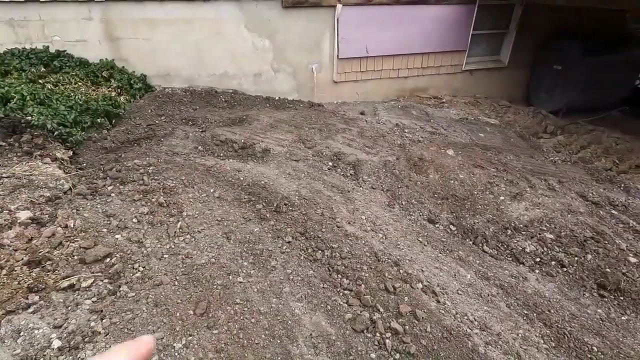 eight feet in depth, i'll use that product. if not, i'll use the backfill material soil with a little rocky soil and i'll compact it in 12 inch lids. so that was about seven tons of the overburden put back. uh, we just put in actually 20 tons. 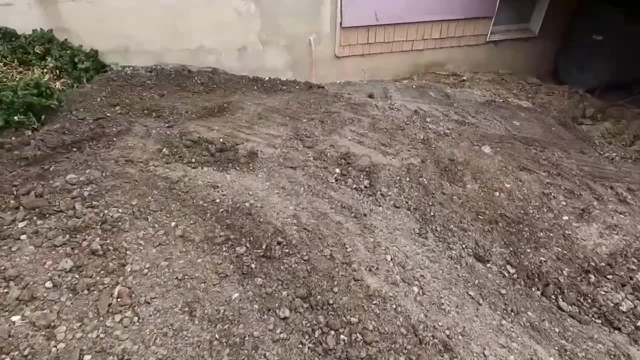 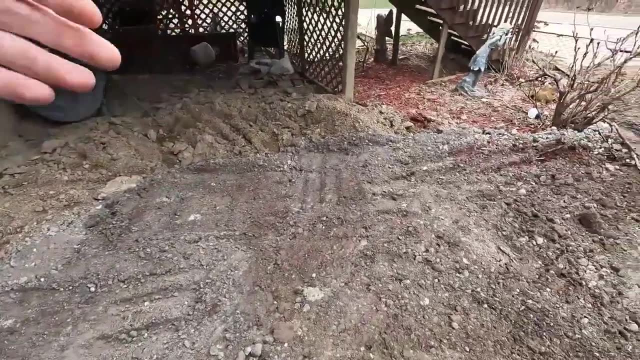 of the item crusher compacted. it's pretty firm right here. we're just going to finish this off by hand and then we'll hand it over to the next person to do the overburden and tamp that we'll rake all the edges in and now we're just going to start coming in with dirt. 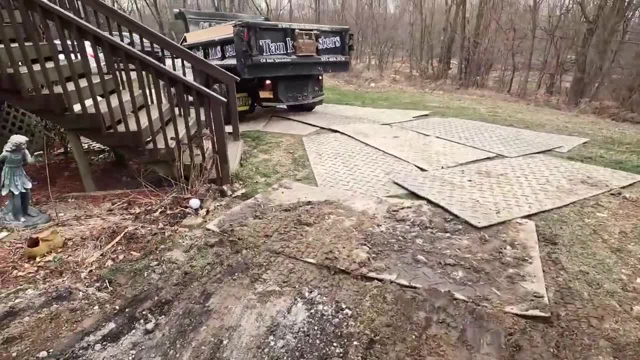 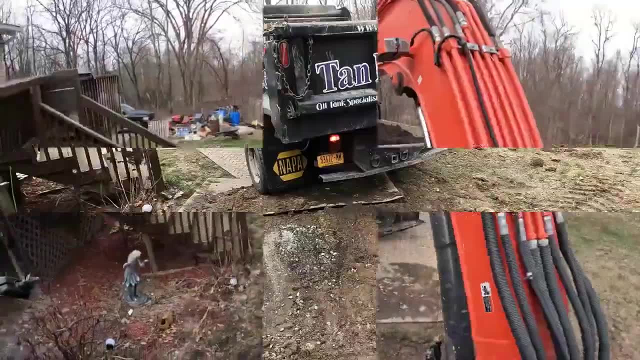 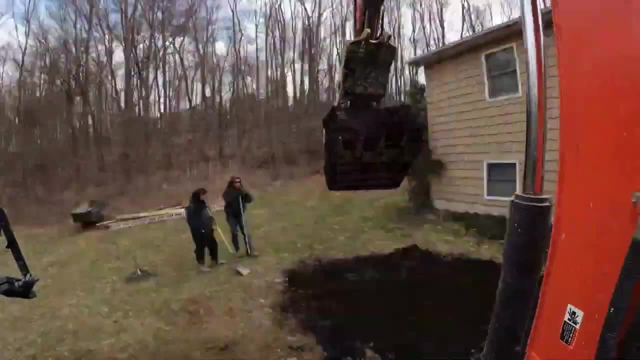 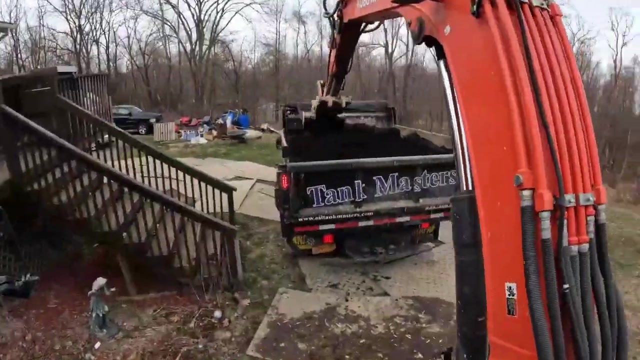 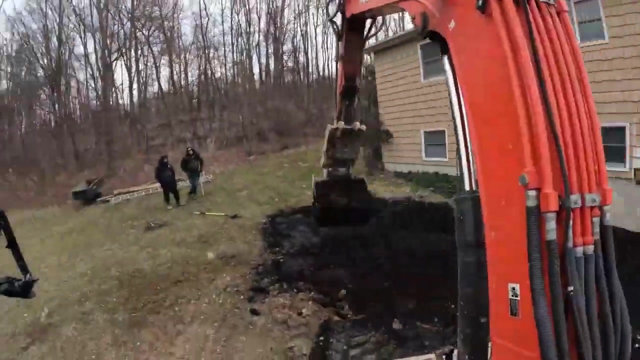 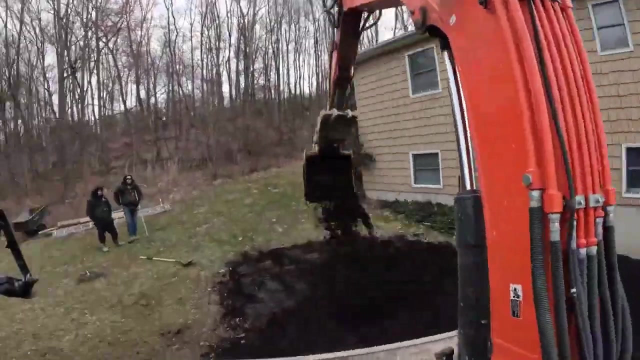 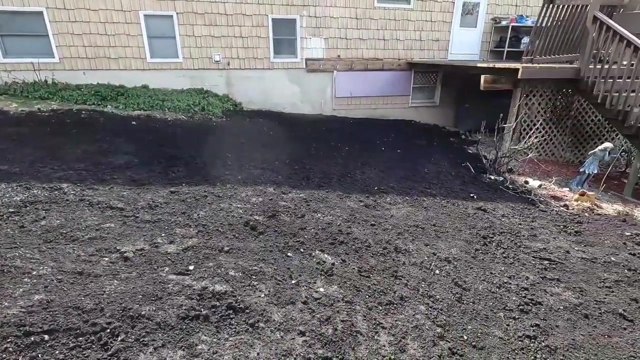 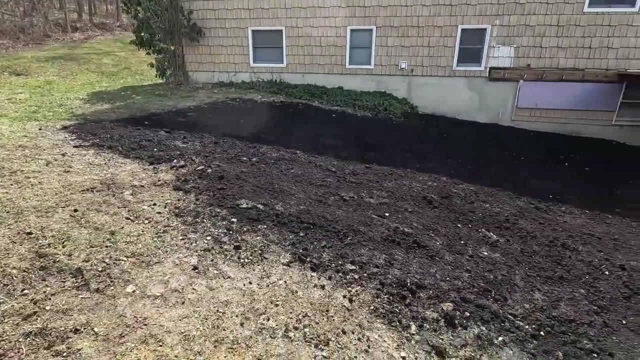 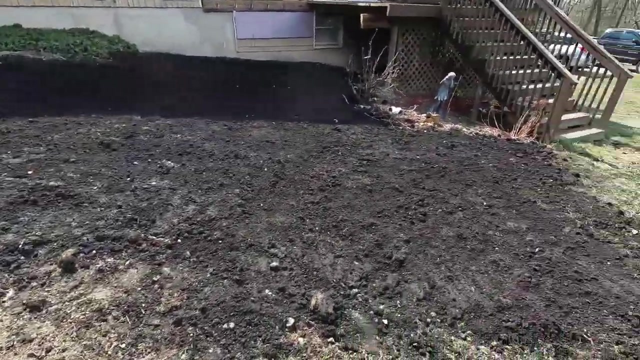 or topsoil. so after we put all the the item crusher in, we compacted that. then we regraded this area where it was loose, compacted it. then we set our topsoil, put a little bit of dirt in there and then put a little little compact on that topsoil and then we rake it out and that's it. that's a finished. 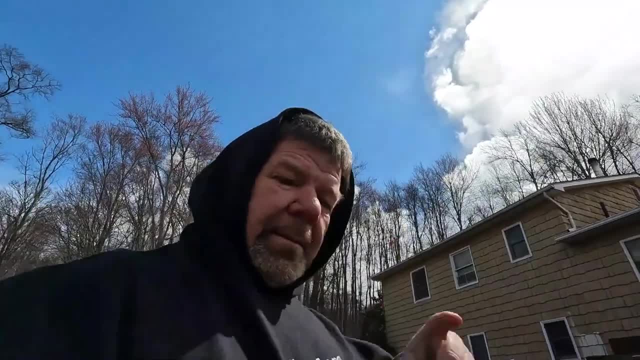 soil remediation by tank masters environmental.